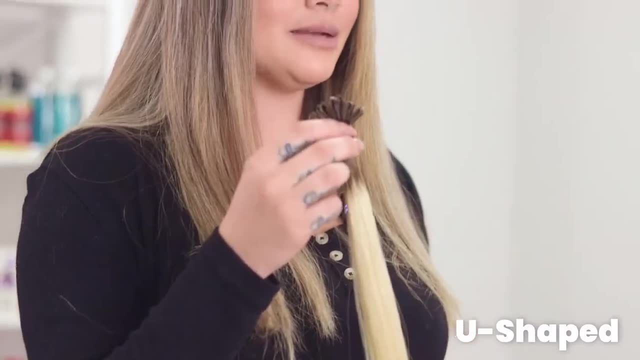 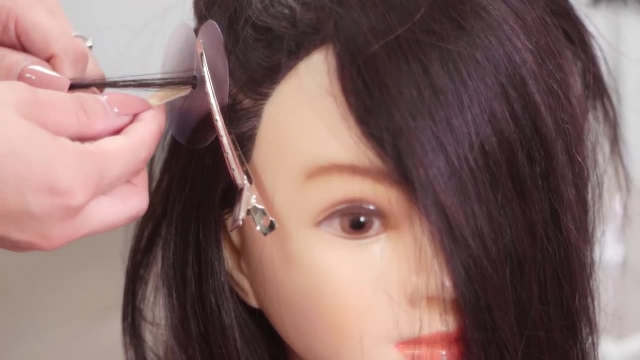 Our nail tips are shaped in a U. Our nail tips require a hot tool. All you really need to do is take a nail tip and bond it and fuse it with your hot tool and the keratin bond And once that's complete, you will have a full set of hair that looks super natural and really, really durable. 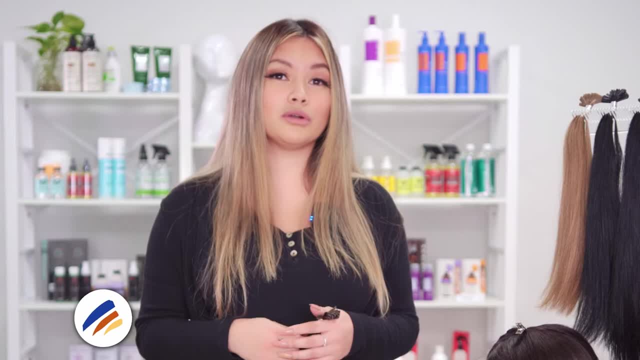 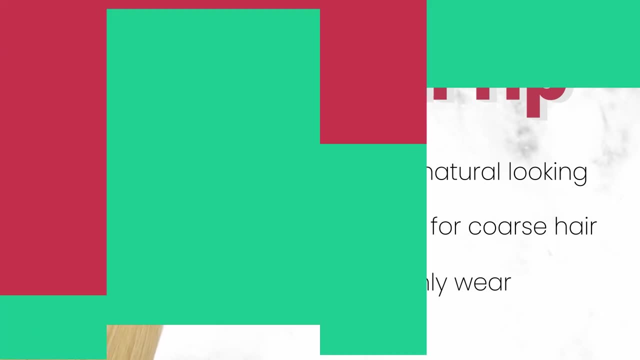 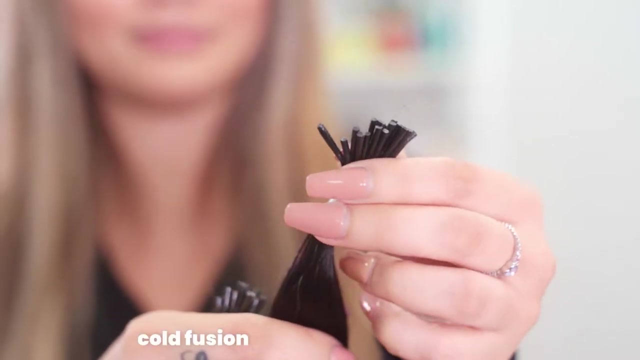 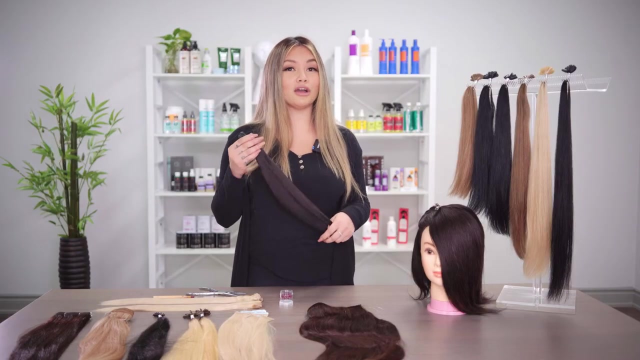 Hot fusions, or our nail tips, are one of our most durable and long-lasting hair extensions. All right, let's talk about eye tips. Eye tips are also known as cold fusions, stick tips or microlinks. They are very easy to attach and also as durable as hot fusion U-tips. 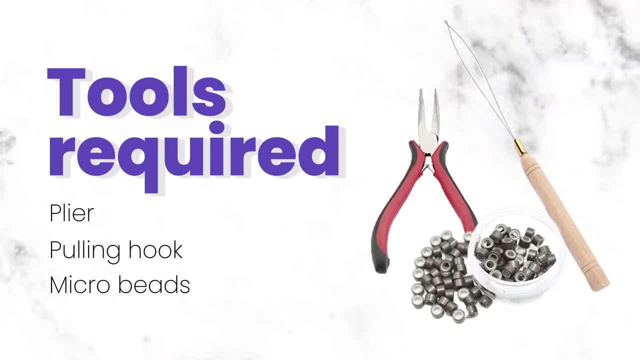 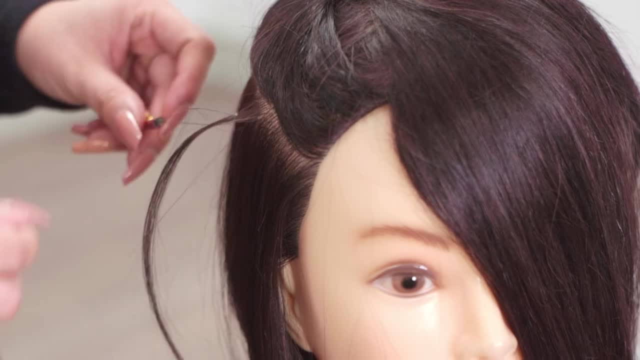 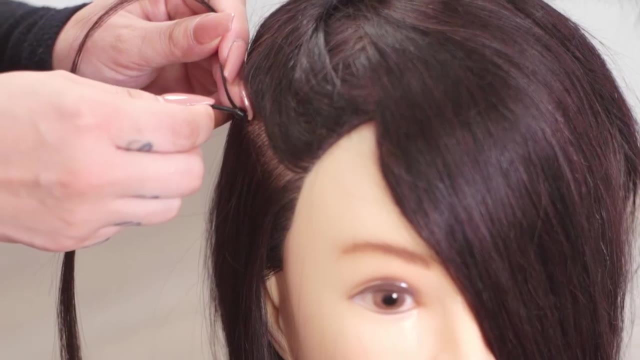 All you need is a plier pulley and some beads. How to attach an eye tip is very easy. You take a strand of hair, pull through the pulley, grab a bead and pull the hair through. Then you're going to take the eye tip and just simply attach it inside. 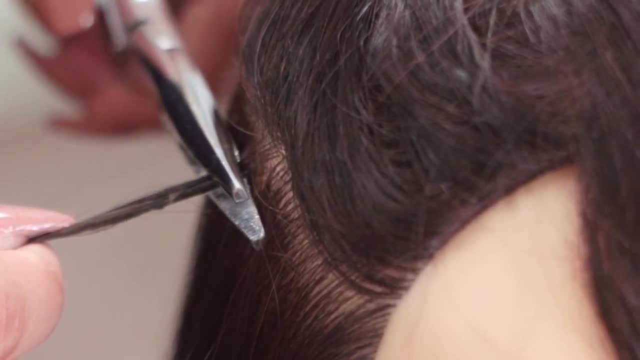 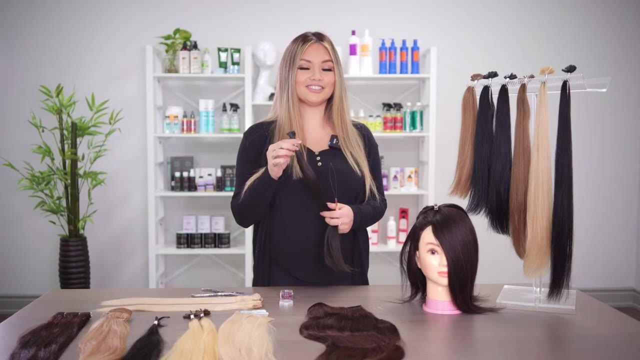 Then take your plier and bond the two together. Eye tips do need to be maintained every three weeks, since the hair growth will pull down the actual hair. For easy access to the scalp with no hot tools required and a durability that will last you for a month, eye tips are the way to go. 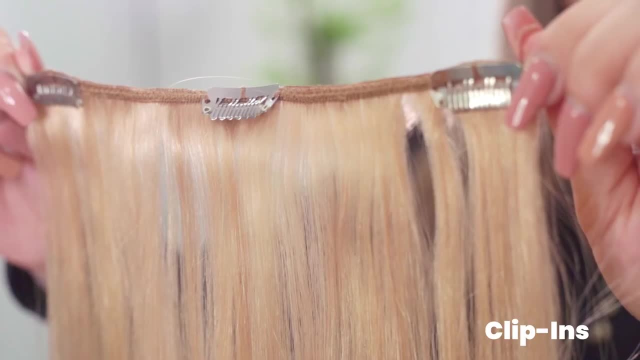 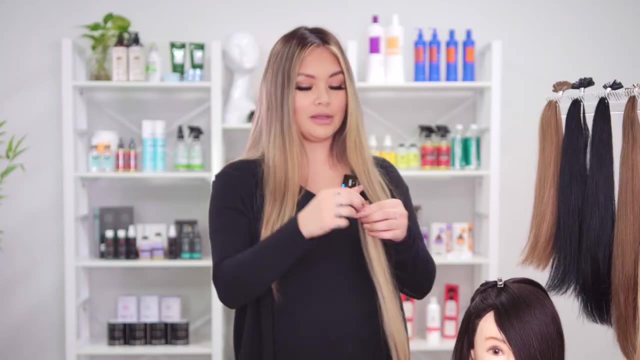 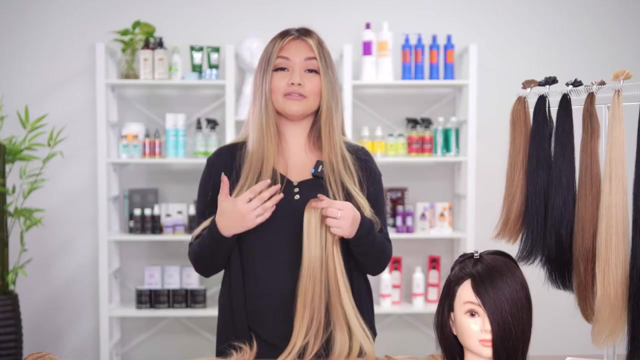 Let's talk about our clip-ins. At Super Hair Pieces we have four long clips, four single clips and as well as two extra pieces just in case. Clip-ins are temporary, easy to install on yourself and on your clients. They also give an instant look and are great for any special events like weddings or just a simple night out. 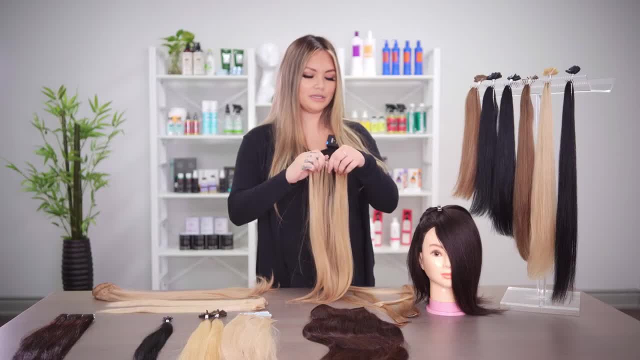 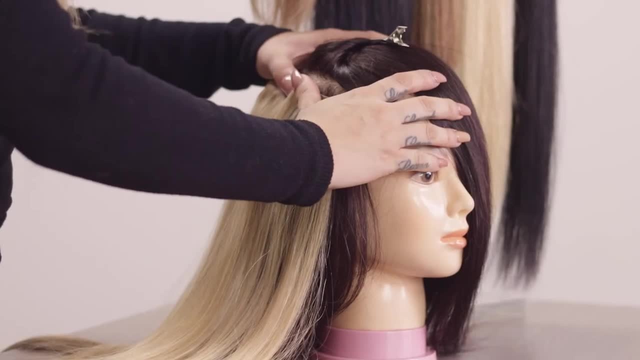 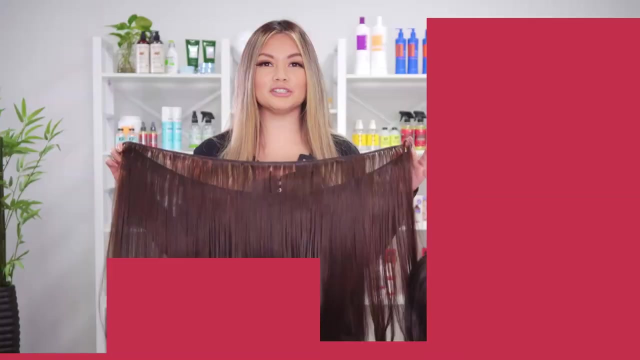 So to put hair clips extensions, it's super, super easy. Take the clip and put it right on to the hair and just clip it on. Super easy, super fast. Machine wefts are voluminous, dense and extra sturdy. 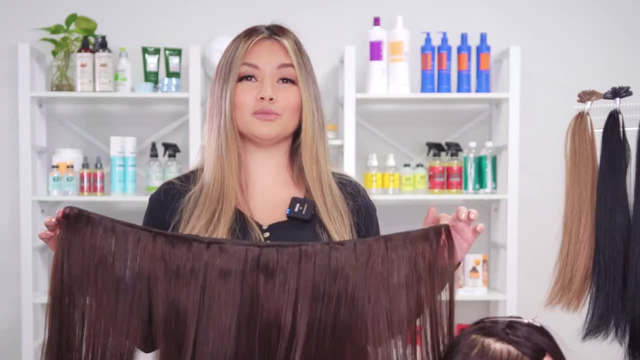 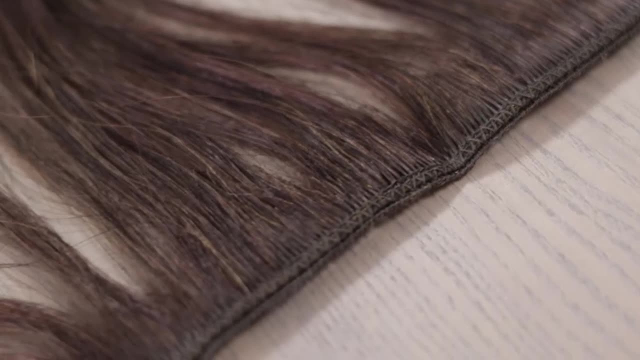 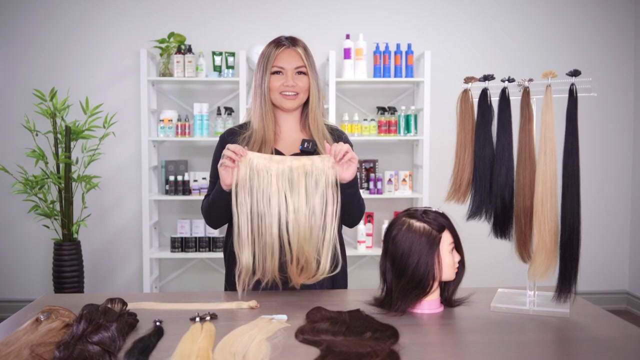 You can use machine wefts for any style you want, and there's different methods of attaching. You can attach it with glue, with beads, or even integrate it with a hair system. The next hair extension I'm going to talk about is our hand-tied wefts.